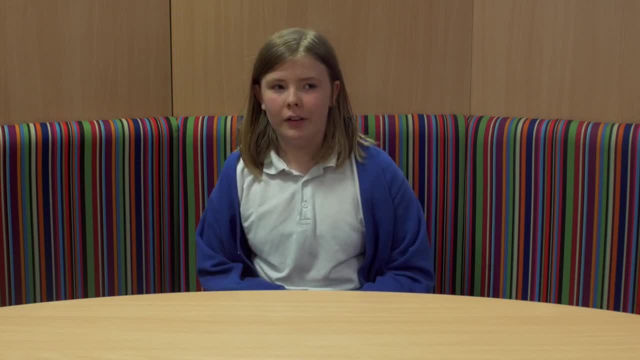 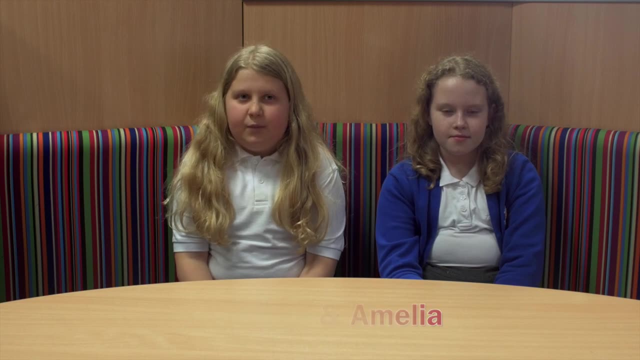 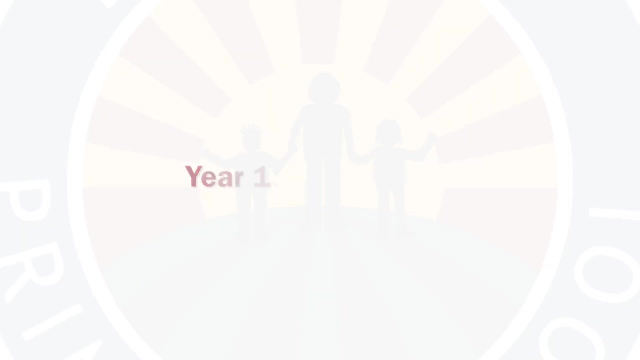 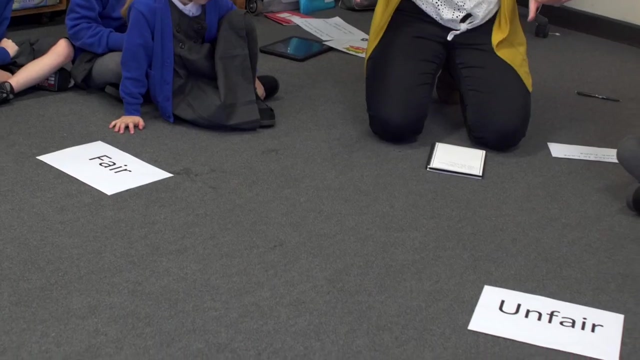 people confidence and we get to talk about stuff that properly matters. P4C is where people are able to collaborate to be able to make decisions on what people's opinions are on different topics. Each partner should now have a statement and you need to decide. is it fair or unfair? 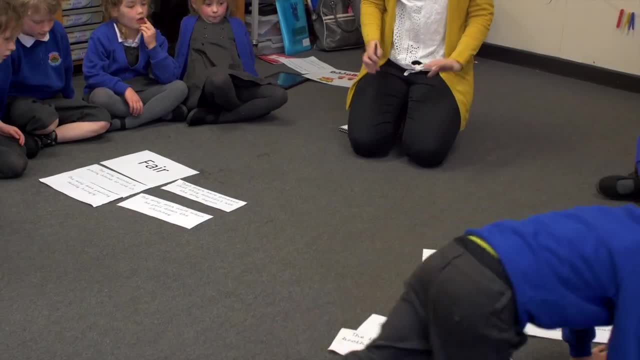 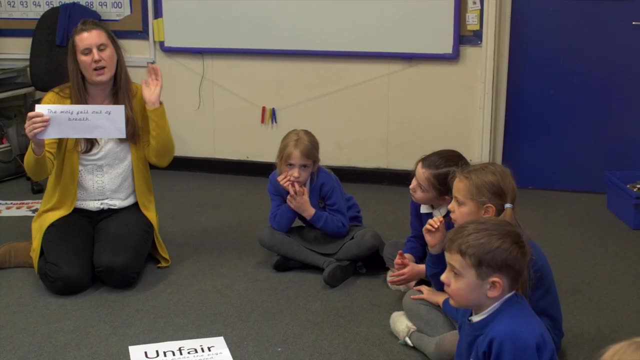 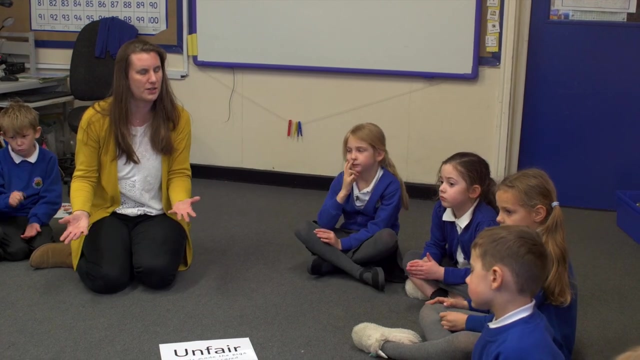 Do you know? what I'm really impressed with is that you have managed to sort them really clearly into fair and unfair. So whoever had this has put that it is unfair that the wolf felt out of breath. Could we even use what we did in our warm up? yes, but to maybe put 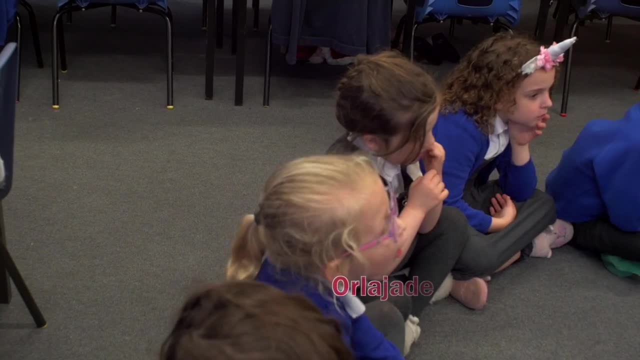 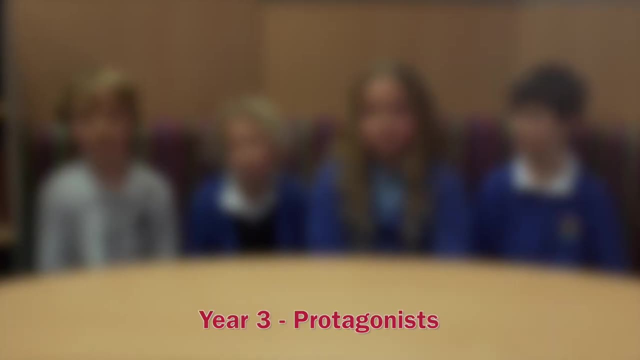 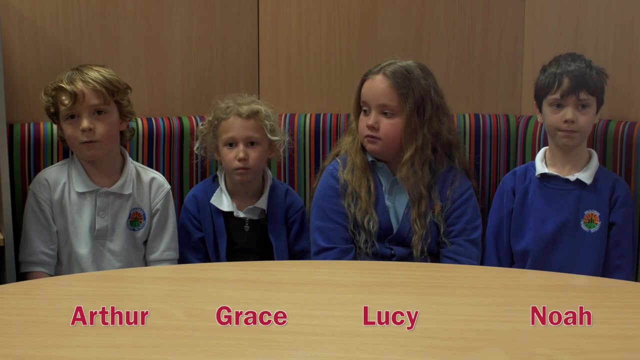 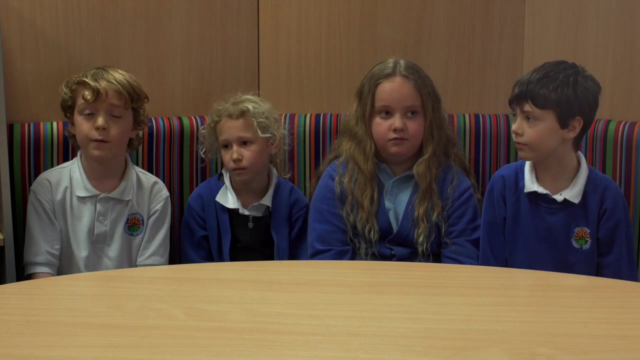 a different idea forward on that one. So that's his own fault for blowing all the houses down- only three houses. We just normally come and sit around in a circle, We watch videos, then we talk about the video and sometimes, when we do the questions, we vote on the questions, Whichever one gets. 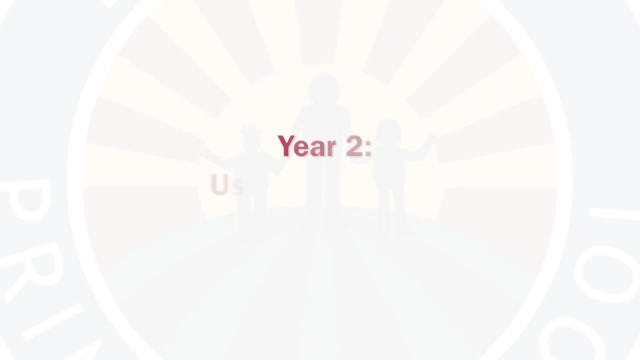 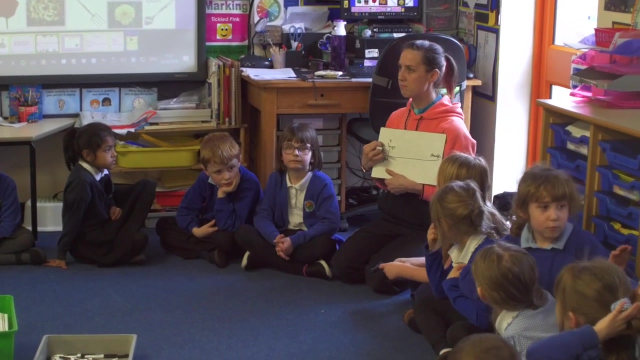 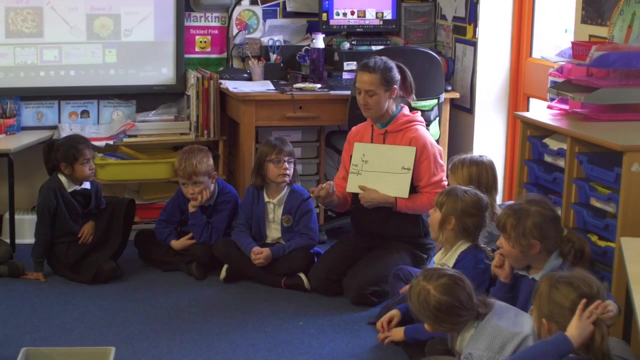 the most votes. then we talk about that one. I could say, like Ray said, they've got no colour, They're just brown and boring. You could find them on the ground and you wouldn't really be interested in a twig. But Olivia might say, no, they're beautiful, they're from a tree, a living thing. 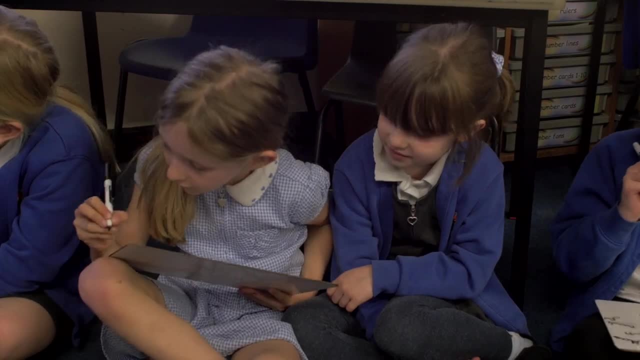 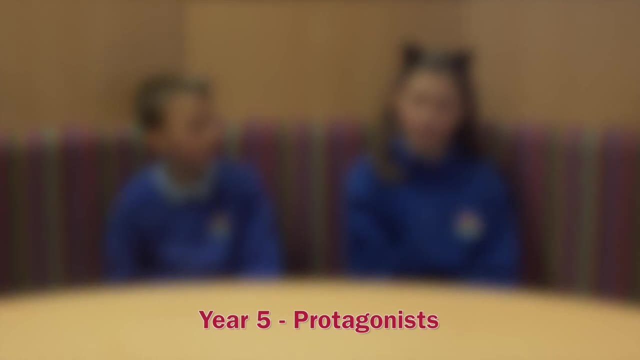 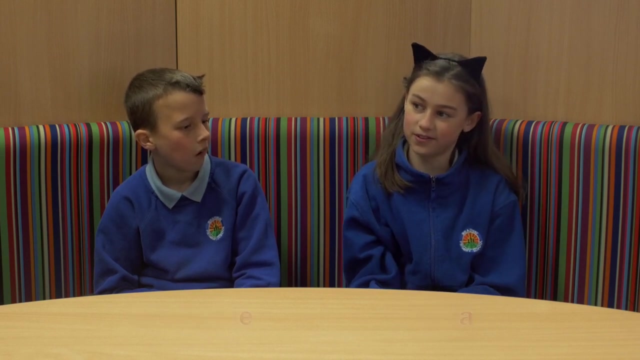 They're able to express opinions, they're able to understand that they may have a different opinion to someone else, and that's okay. We do this thing where the teacher claps and we have to try and clap at the exact same time all together. 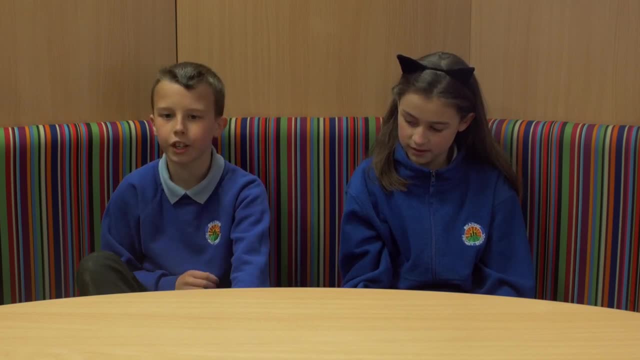 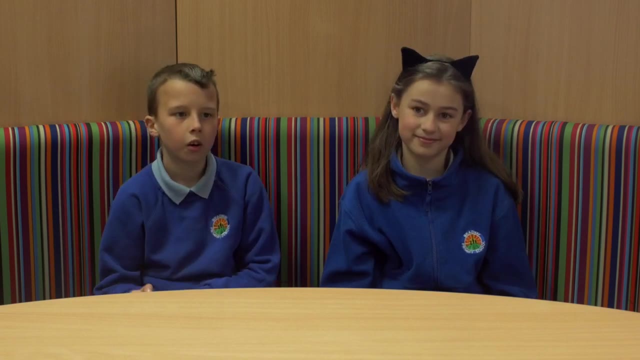 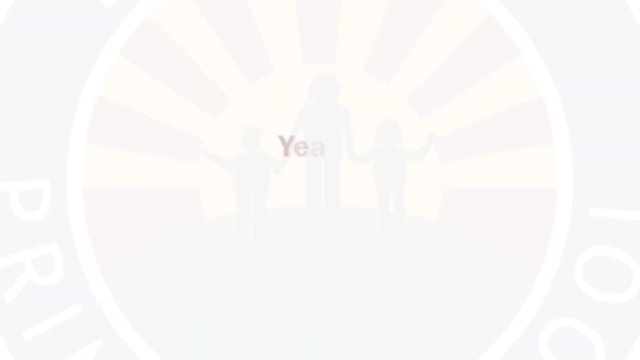 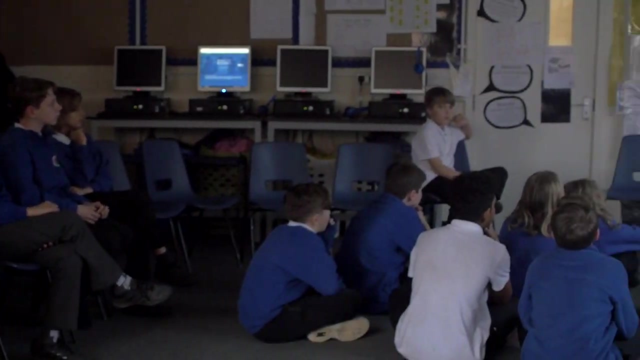 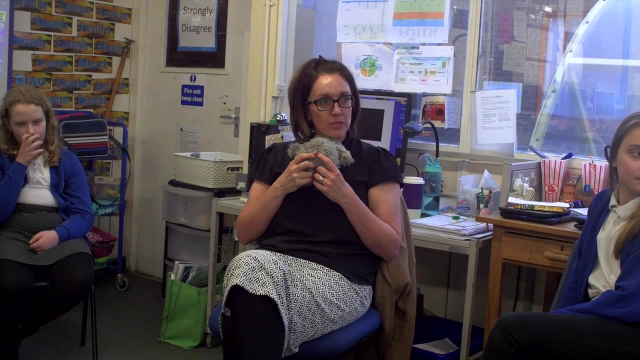 And that's to help to see if we're concentrating. We had someone called Nick in and he did it with us. A boy called Hugh was concentrating really well, It was like he was reading his mind. Has anyone got a response or a first thought about that question, about what is beauty? 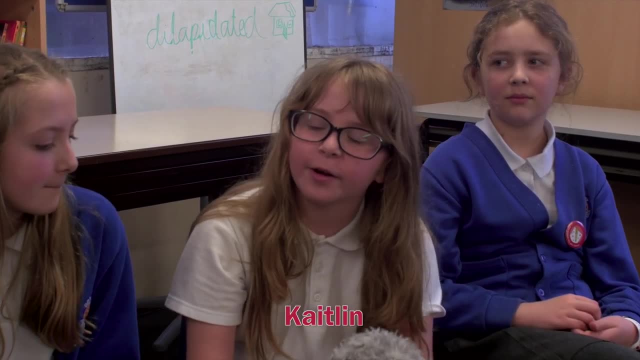 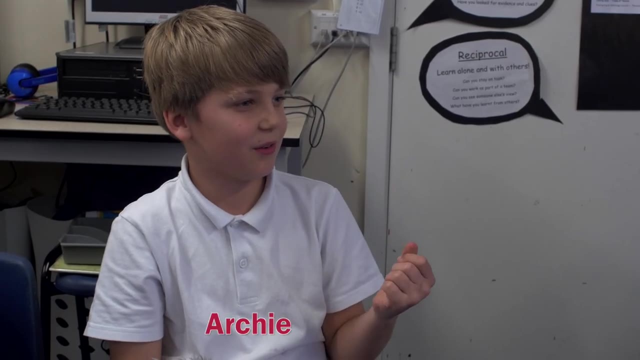 You can be beautiful if you're beautiful. You can be beautiful if you're a boy or a girl. So it's really not a girl is beautiful, It can be both. Not everybody has to see you as beautiful, But beauty is in the eye of the beholder. What does it mean?